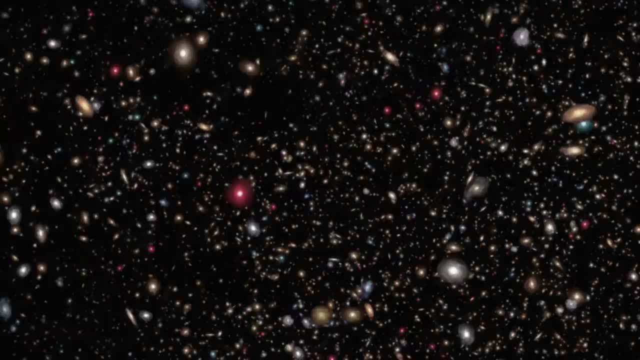 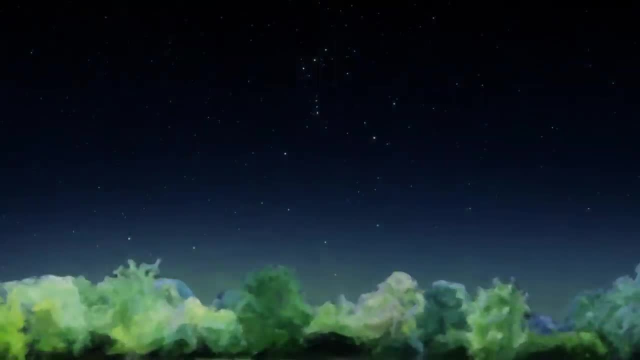 Cities of billions of stars, and more than a thousand of them are hidden behind your thumb. The universe is bigger than you can see from the city and even bigger than the starry sky you can see from the countryside. This is the universe as astrophysicists. 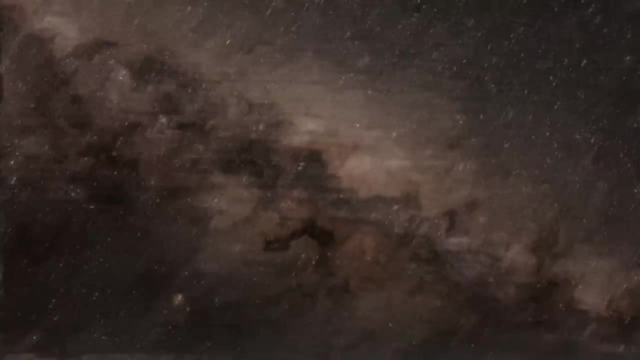 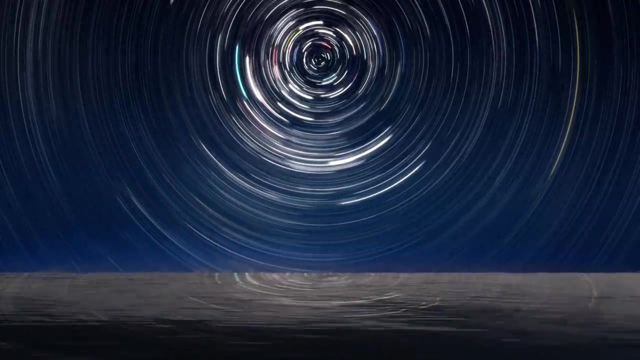 or, as physicists see it, with more stars than all the grains of sand on Earth. By staring up at the stars at night, you've taken part in the oldest science in human history. The study of the heavens is older than navigation agriculture. 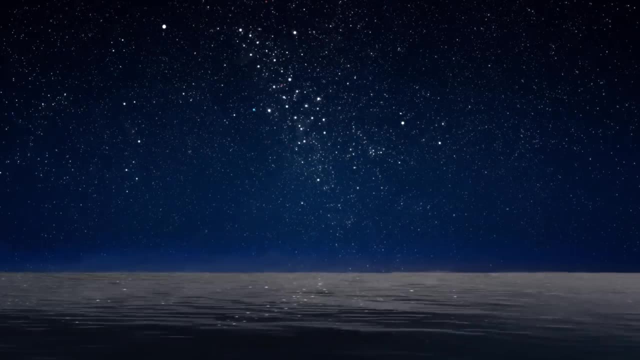 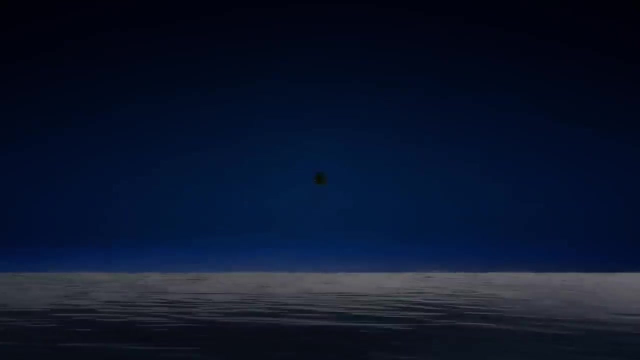 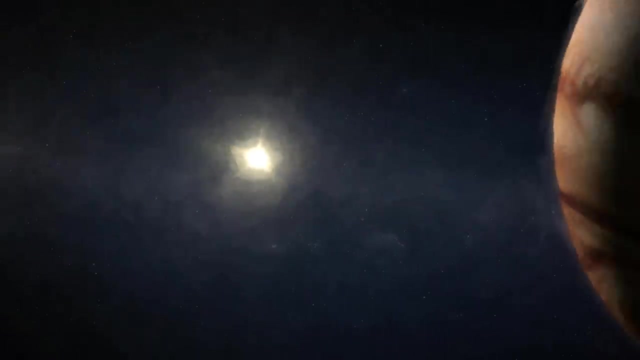 perhaps even language itself. Yet, unlike other sciences, astronomy is purely observational. We cannot control the parameters of our experiments from lab benches. Our best technology can send man to the moon and probes to the edge of the solar system, But these distances are vanishingly small compared to the yawning gulfs between stars. 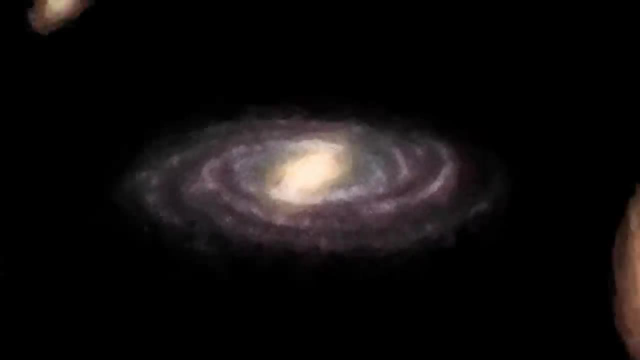 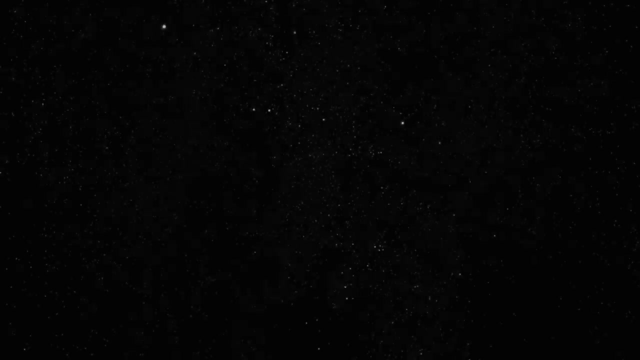 So how can we know so much about other galaxies, what they're made of, how many there are, or that they're even there at all? Well, we can start with the first thing we see when we look up at night: the stars. 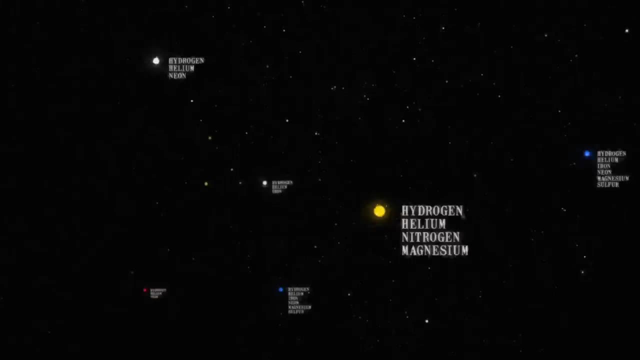 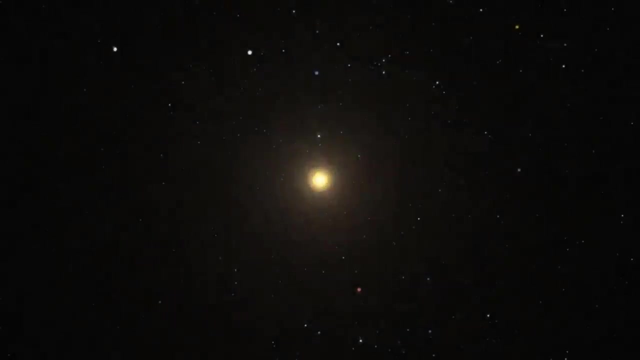 What we are trying to learn is their properties. What are they made of, How hot are they, How massive, How old, How far are they from Earth? And, believe it or not, we can learn all of these things simply from the light shining in the sky. 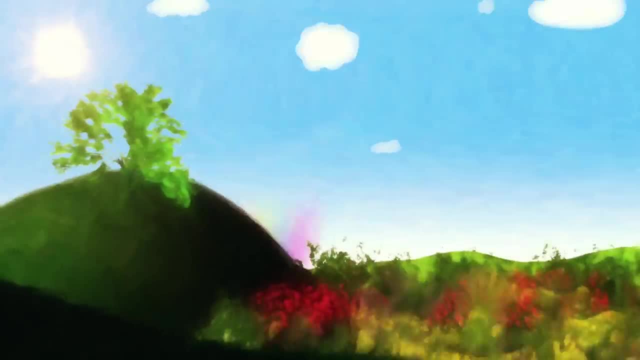 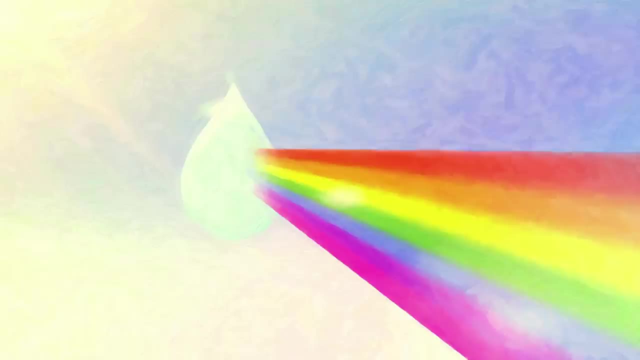 We can decipher one kind of stellar message by turning starlight into rainbows. When you look at a rainbow on Earth, you're really looking at light from our sun being scattered through water droplets in the atmosphere into all the different wavelengths that make it up. 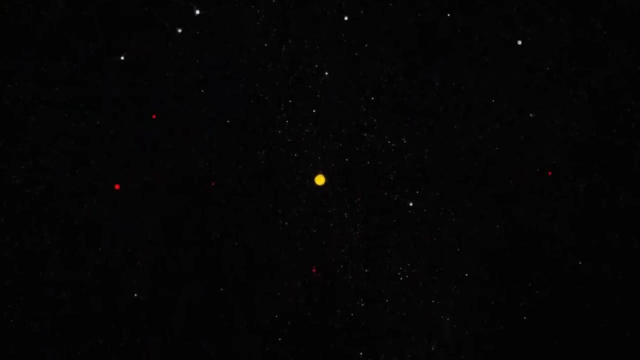 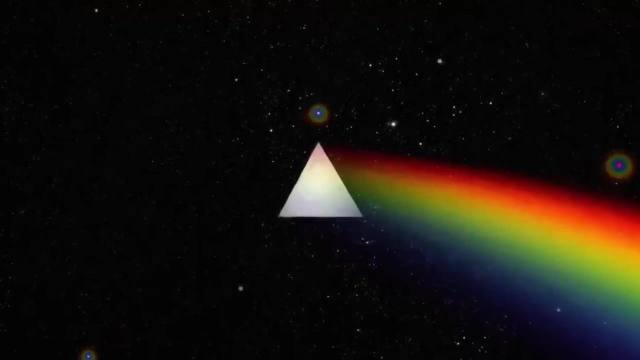 And when we study the light from other stars, we can create rainbows on demand using not water droplets but other specific instruments that disperse light. When we look at the scattered light from our sun, we see something strange: dark lines in our rainbow. 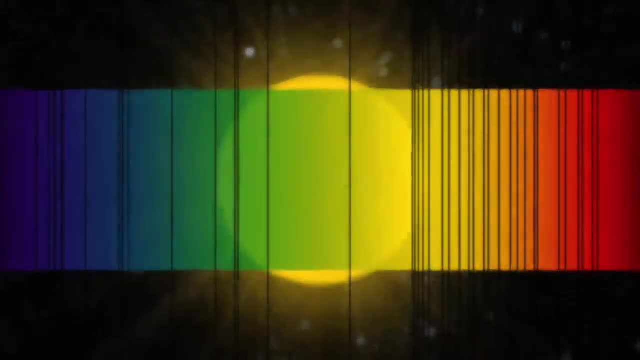 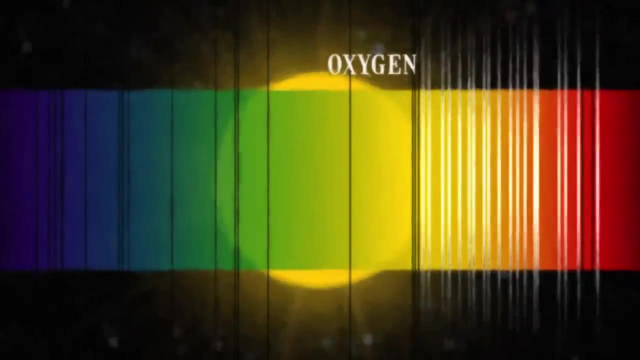 These lines are the characteristic fingerprints of atoms. Each type of atom in the solar atmosphere soaks up light at specific wavelengths, and the amount of absorption depends on how many of these atoms there are. So, by observing how much light is missing at these characteristic wavelengths,